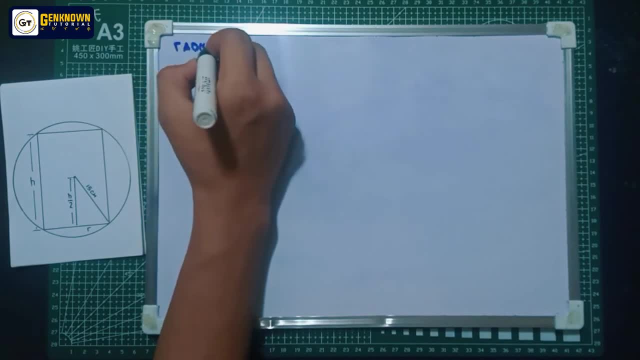 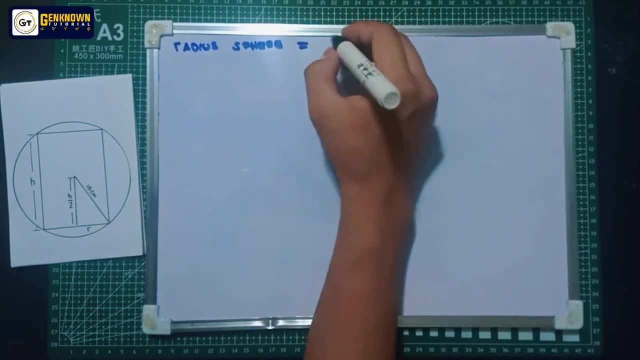 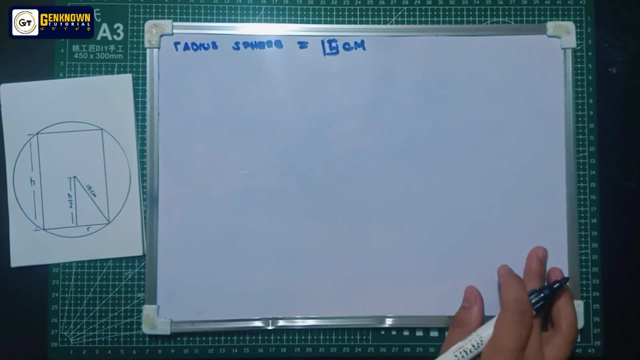 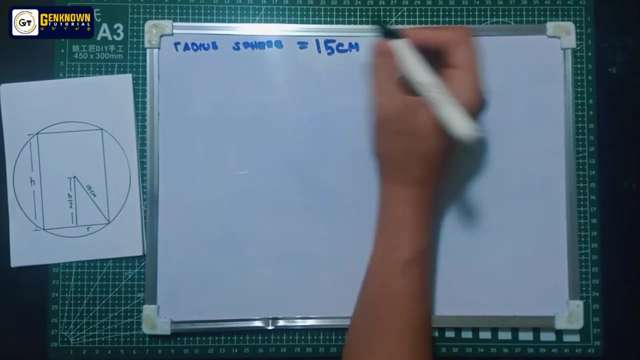 Please subscribe to my channel and press the bell icon. Please subscribe to my channel and press the bell icon. Excuse me for the background noise, but you may be able to hear those background noises correctly. Next I make a'mos life shake. 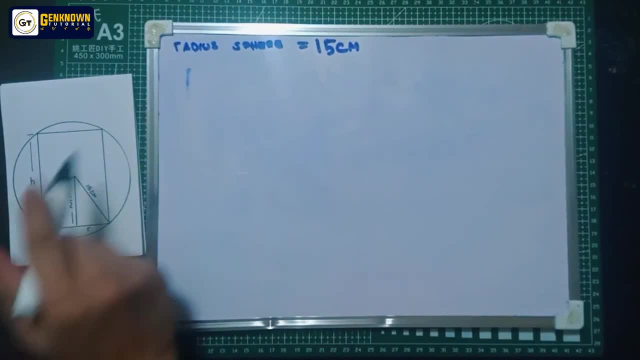 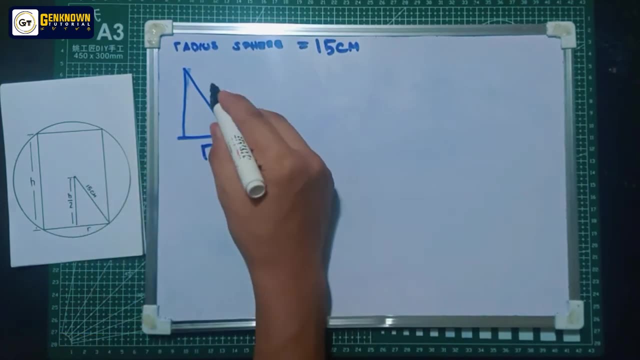 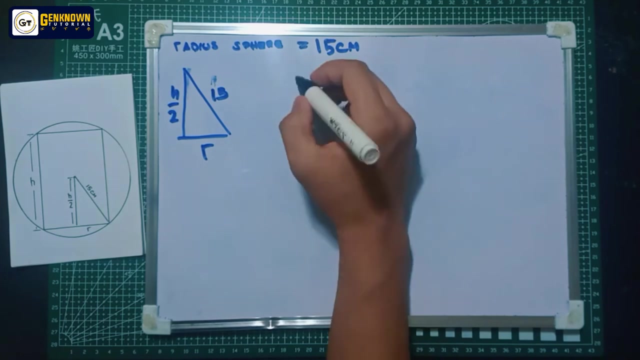 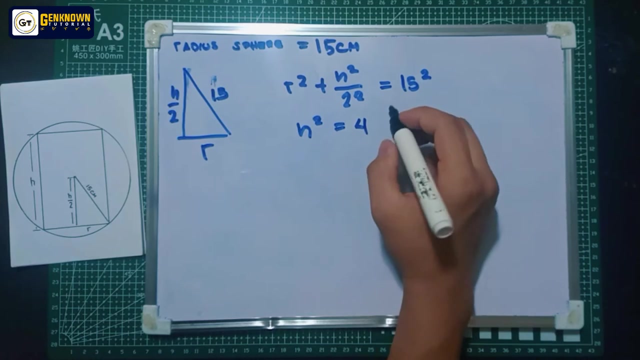 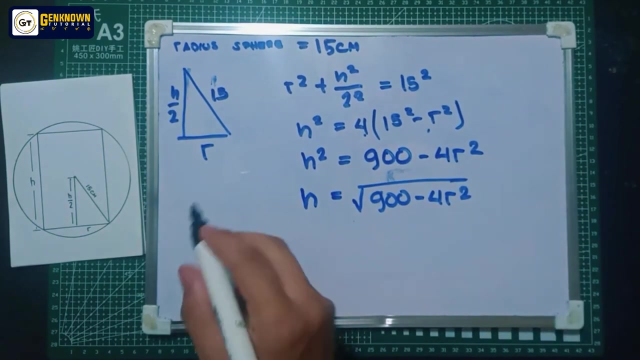 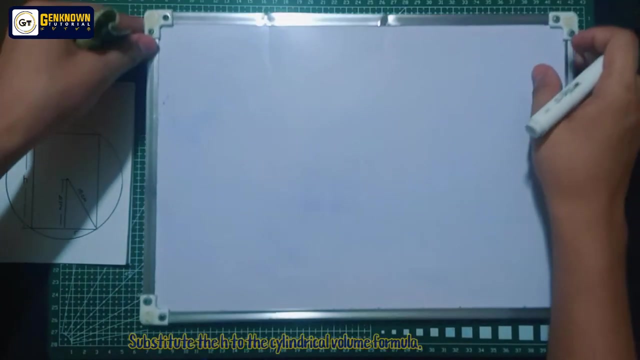 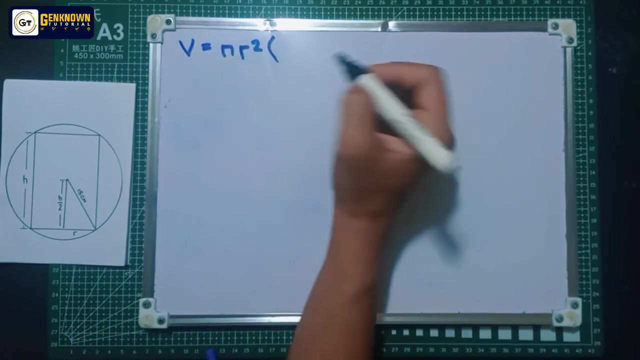 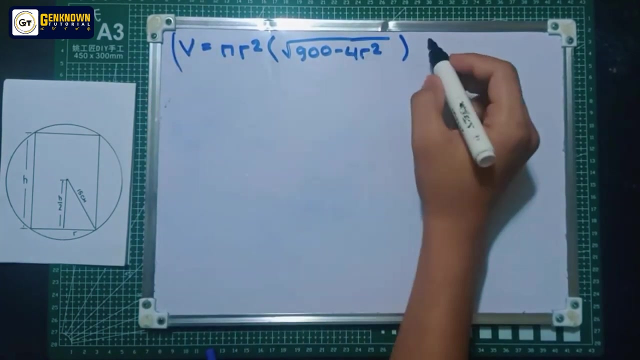 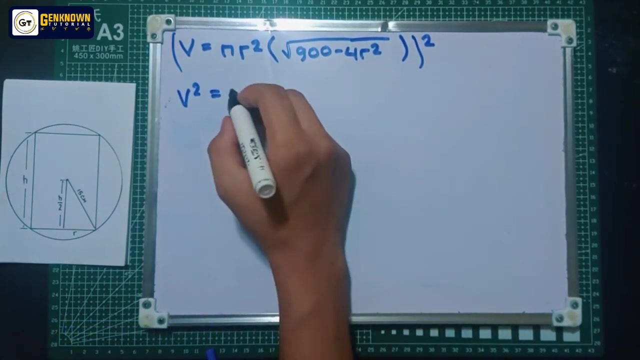 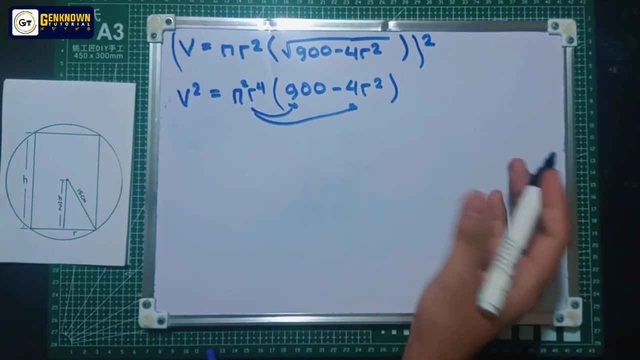 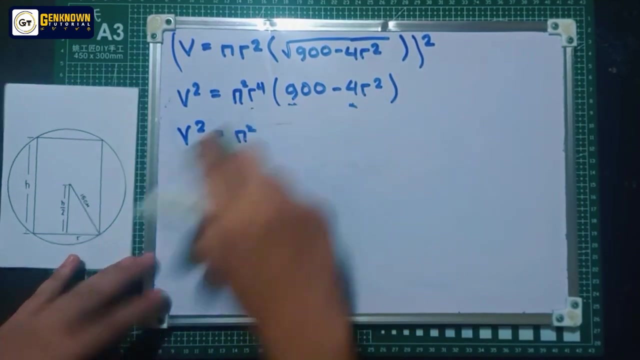 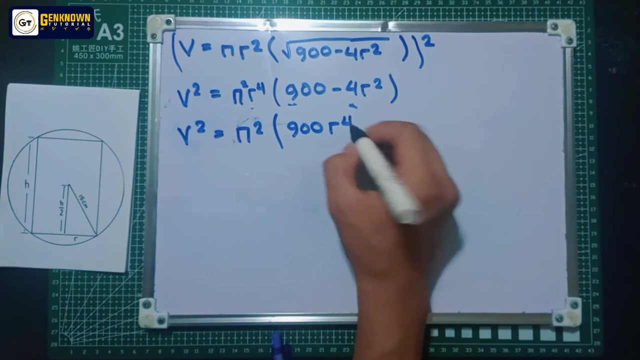 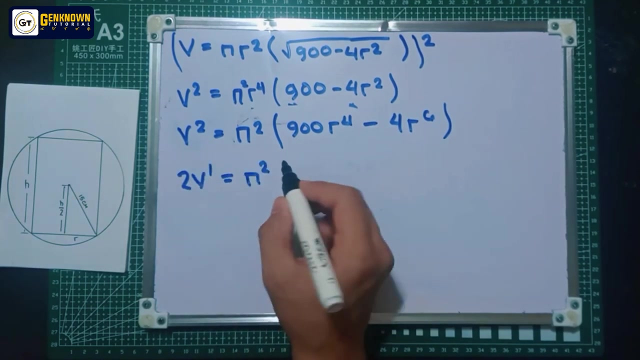 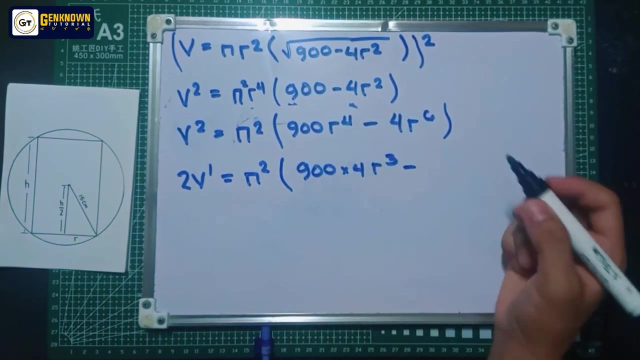 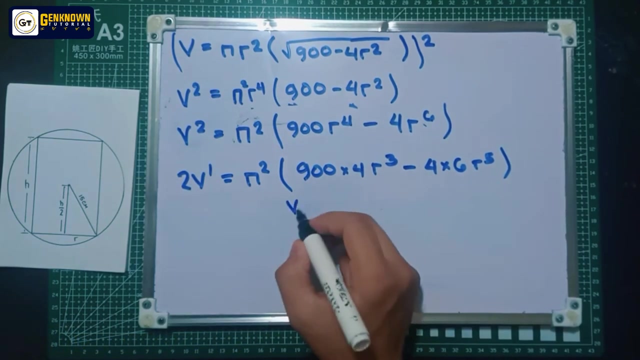 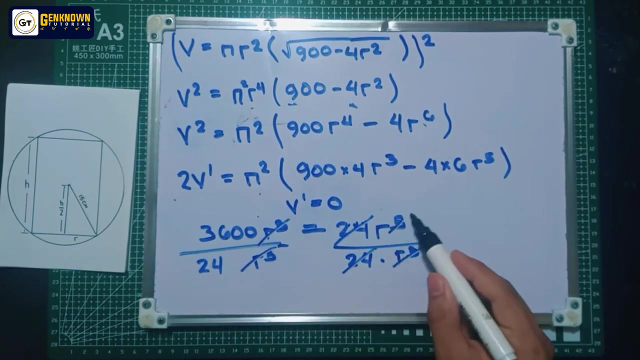 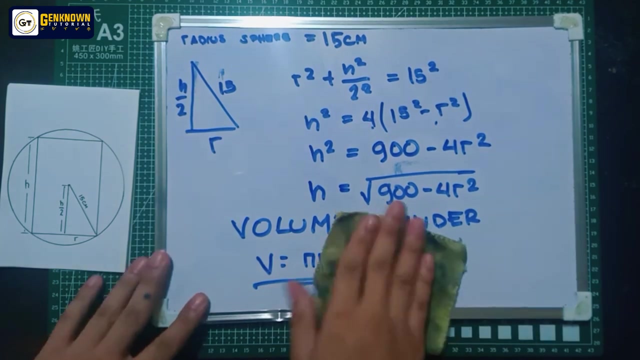 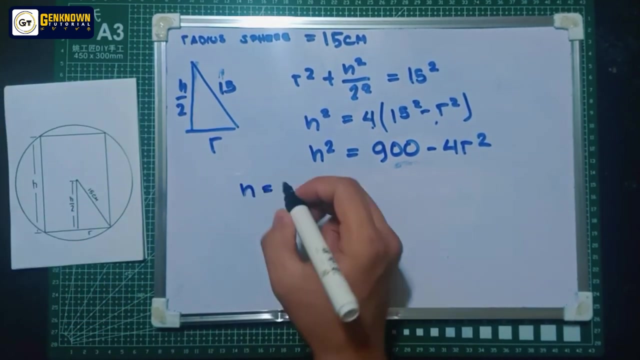 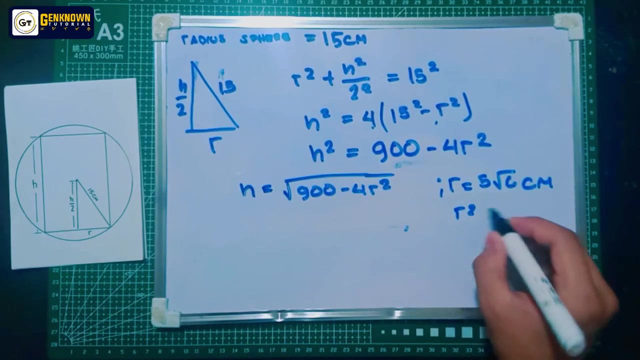 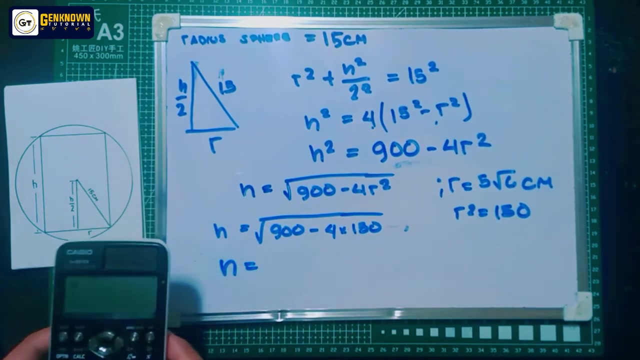 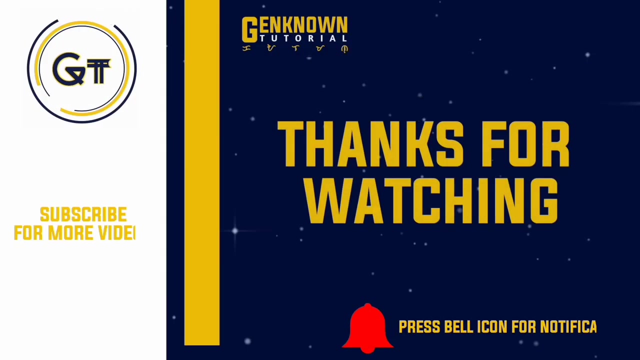